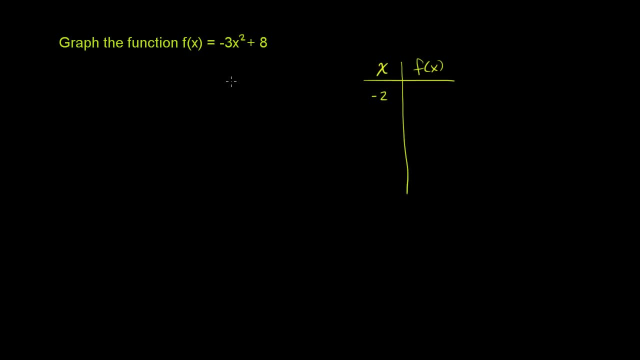 it's probably going to be a curve, the generalized shape of the curve, And then I can continue. I'm going to connect the dots. So, when x is negative 2, what is f of x? f of x is negative 3 times negative 2 squared plus 8,. 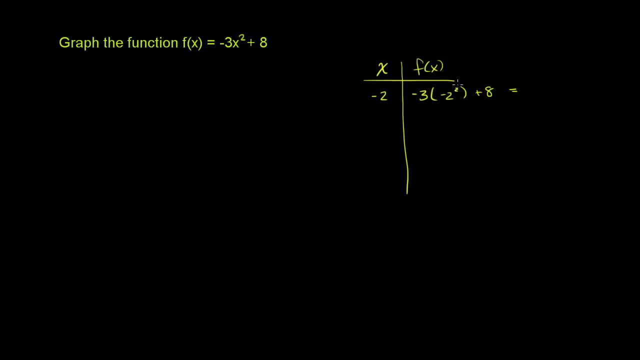 which is equal to negative 2 squared is positive 4.. Positive 4 times negative: 3,. let me write this: is negative 3 times 4 plus 8.. That's negative 12 plus 8, which is equal to negative 4.. 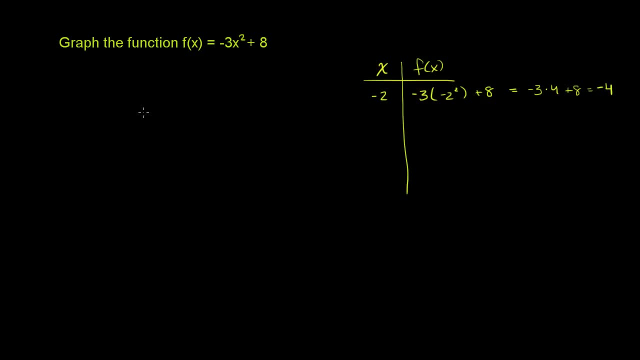 So the point negative 2, negative 4 is going to be on our graph. Actually, let me just start graphing it. So let me draw my, I'll call this the y-axis And I'm just going to set our y values, whatever. 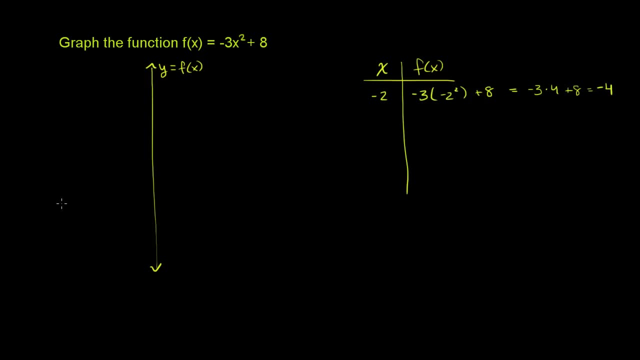 the output of our function is So: y is equal to f of x. And then let me draw the x-axis. So let me draw the x-axis like this. So let me draw which. I want to do it like this. I'll draw the x-axis like that. 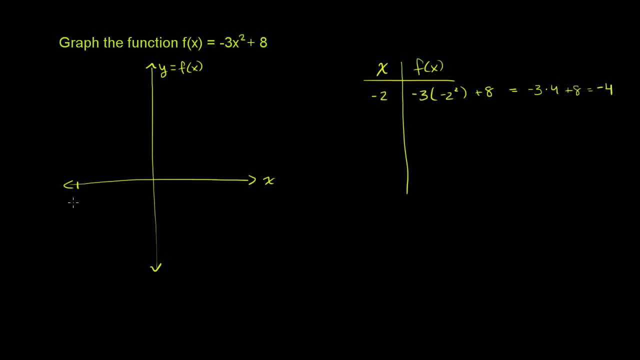 So there's my x-axis And I'm going to try the points: x is equal to negative 2, x is equal to negative 1, x is equal to 0, x is equal to 1, and x is equal to 2.. 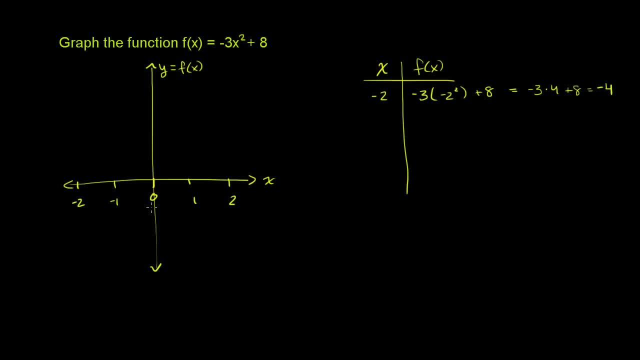 So this first point over here- 2, negative 4, and actually let me graph that. So let's say that this right over here is negative 4.. This would be positive 4.. And this would be positive 8.. So the first point is negative: 2, negative 4.. 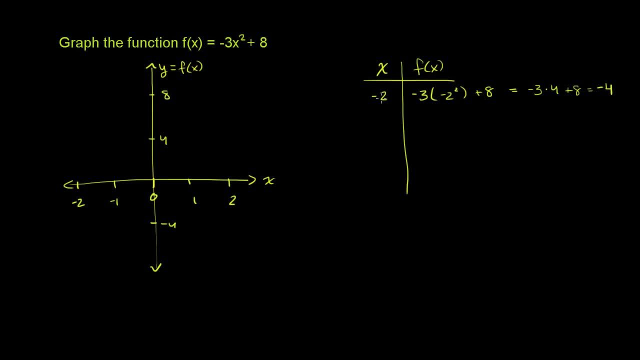 When x is negative, 2, f of x, When the input into our function is negative 2, the output is negative 4.. Negative 2, negative 4.. Right over there, That's the point. negative 2 comma, negative 4.. 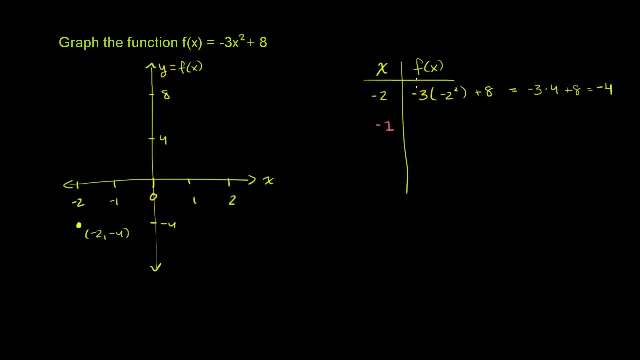 Let's do another one. What happens when x is equal to negative 1?? Then f of x is negative 3 times negative 1 squared. Let me write it: Negative 1 squared plus 8.. Negative 1 squared is just 1.. 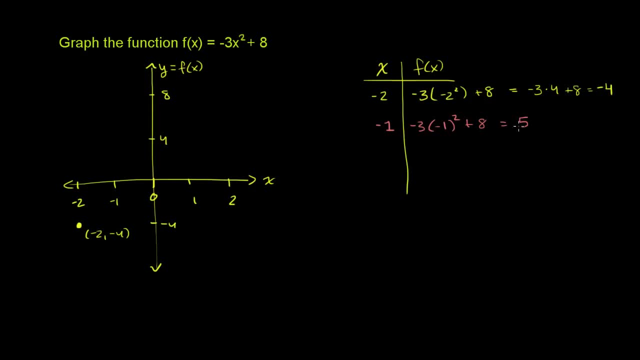 So it becomes negative 3 plus 8. This is going to be equal to 5.. So we have the point negative 1, 5 on our graph, Negative 1, 5.. So this would be 6 right over here. 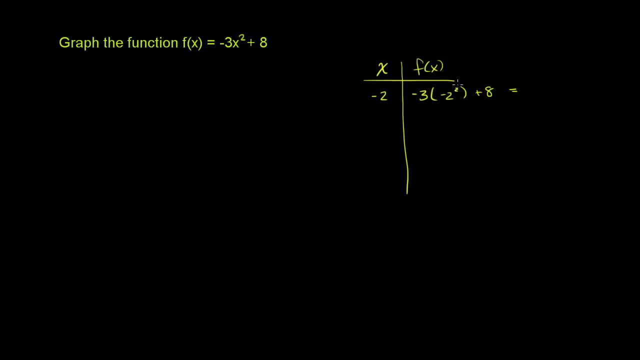 which is equal to negative 2 squared is positive 4.. Positive 4 times negative: 3,. let me write this: is negative 3 times 4 plus 8.. That's negative 12 plus 8, which is equal to negative 4.. 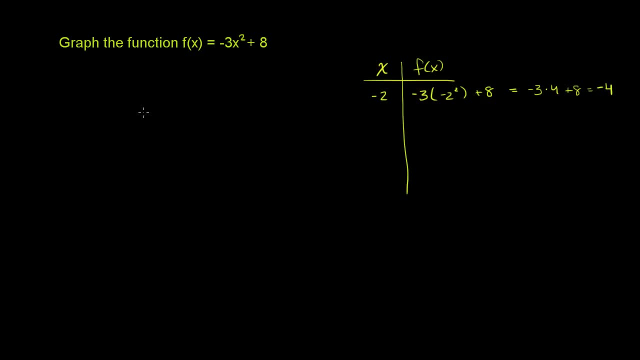 So the point negative 2, negative 4 is going to be on our graph. Actually, let me just start graphing it. So let me draw my, I'll call this the y-axis And I'm just going to set our y values, whatever. 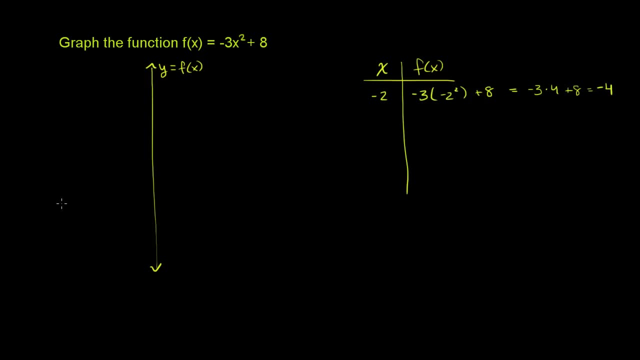 the output of our function is So: y is equal to f of x. And then let me draw the x-axis. So let me draw the x-axis like this. So let me draw which. I want to do it like this. I'll draw the x-axis like that. 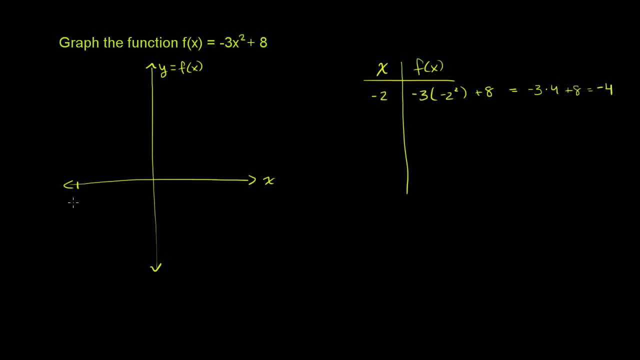 So there's my x-axis And I'm going to try the points: x is equal to negative 2, x is equal to negative 1, x is equal to 0, x is equal to 1, and x is equal to 2.. 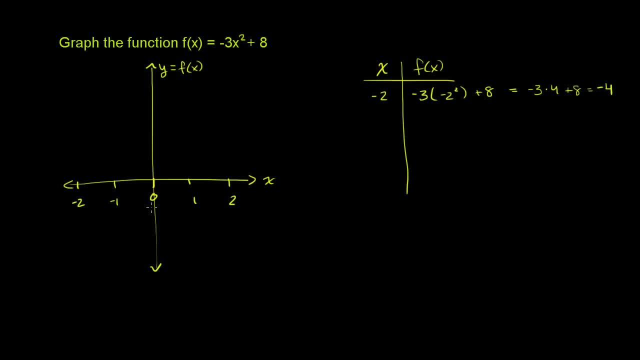 So this first point over here- 2, negative 4, and actually let me graph that. So let's say that this right over here is negative 4.. This would be positive 4.. And this would be positive 8.. So the first point is negative: 2, negative 4.. 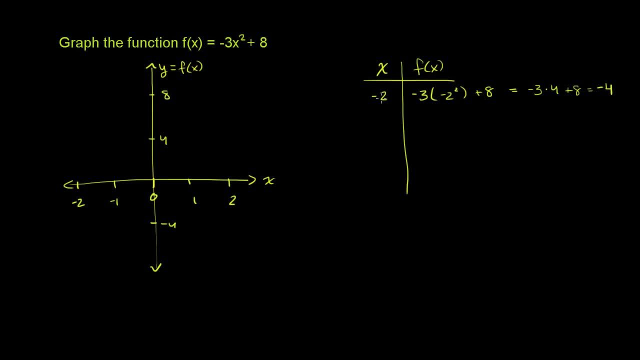 When x is negative, 2, f of x, When the input into our function is negative 2, the output is negative 4.. Negative 2, negative 4.. Right over there, That's the point. negative 2 comma, negative 4.. 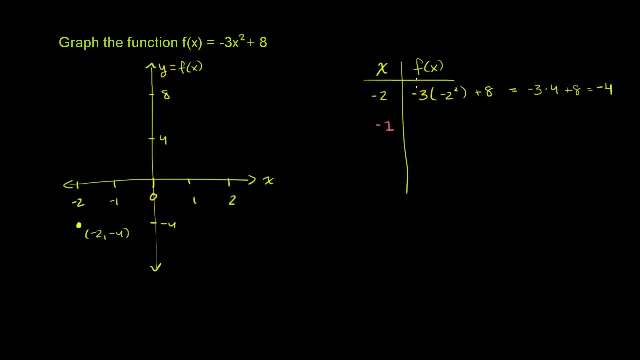 Let's do another one. What happens when x is equal to negative 1?? Then f of x is negative 3 times negative 1 squared. Let me write it: Negative 1 squared plus 8.. Negative 1 squared is just 1.. 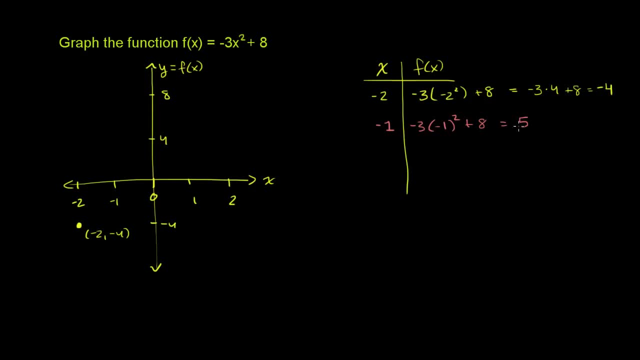 So it becomes negative 3 plus 8. This is going to be equal to 5.. So we have the point negative 1, 5 on our graph, Negative 1, 5.. So this would be 6 right over here. 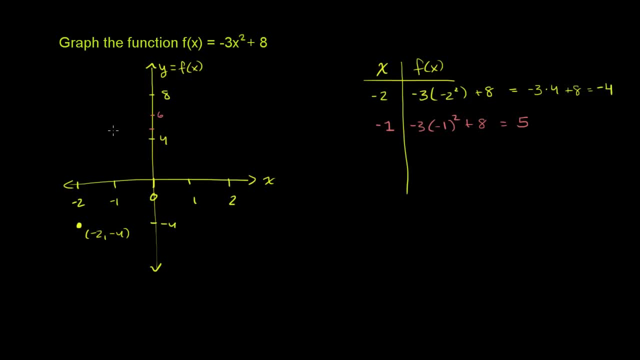 So 5 is going to be right over there. So we have negative 1, negative 1,, 5 is going to be right over there. Negative 1 comma 5.. And then let's see what happens when x is equal to 0.. 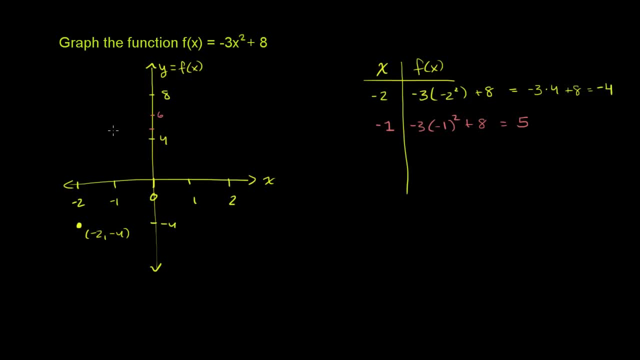 So 5 is going to be right over there. So we have negative 1, negative 1,, 5 is going to be right over there. Negative 1 comma 5.. And then let's see what happens when x is equal to 0.. 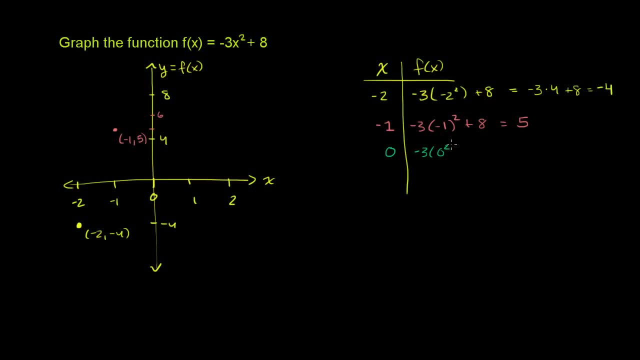 When x is equal to 0, f of x is negative 3 times 0 squared plus 8.. This part's just a 0. So it just equals 8.. So we have the point 0, 8.. 0, 8 is right over there. 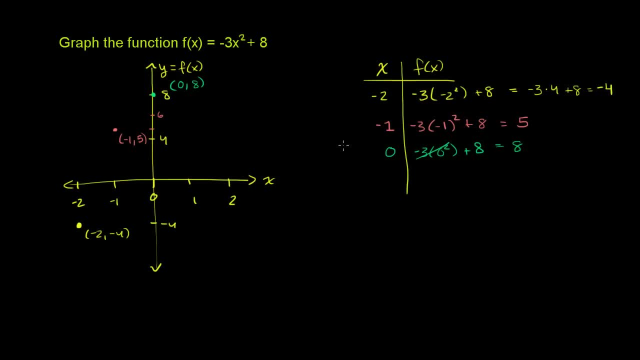 So that's 0.. 0 comma 8.. And then let's see what happens when x becomes positive 1. Then you have negative 3 times positive 1 squared plus 8.. Positive 1 squared is the same thing as negative 1 squared. 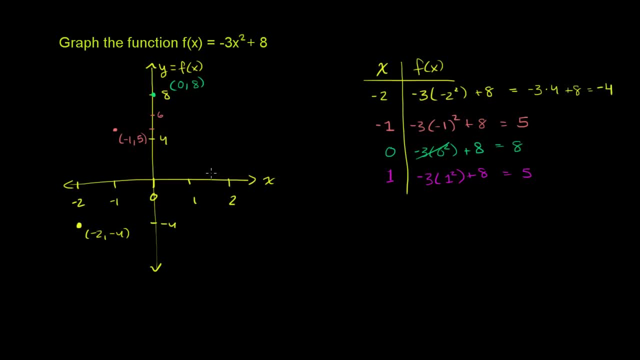 So once again, you get negative 3 plus 8. It is equal to 5.. So this is the point right over here: It is 1 comma 5.. And then, finally, let's do one more point. Let's see what happens when x is positive 2.. 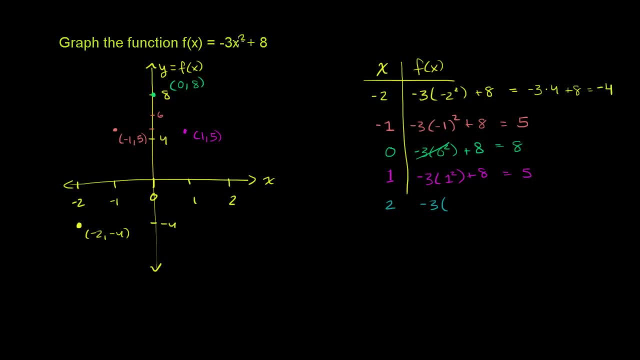 When x is positive, 2, f of x is negative 3.. Negative 3 times positive: 2 squared plus 8.. This, right over here, is negative 3 times 4, which is negative. 12 plus 8 is equal to negative 4.. 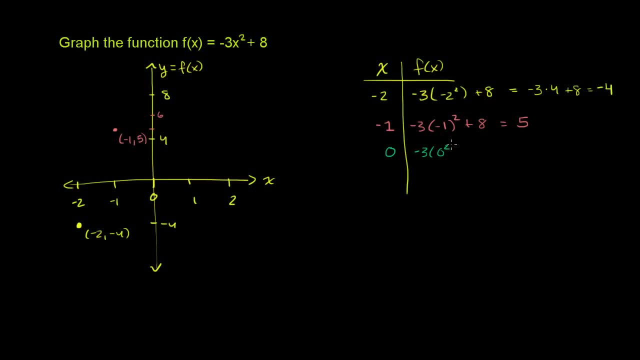 When x is equal to 0, f of x is negative 3 times 0 squared plus 8.. This part's just a 0. So it just equals 8.. So we have the point 0, 8.. 0, 8 is right over there. 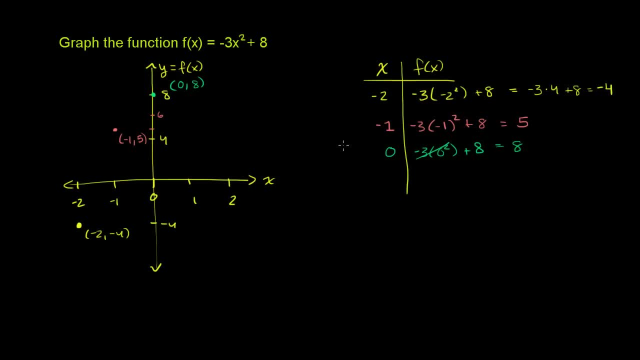 So that's 0.. 0 comma 8.. And then let's see what happens when x becomes positive 1. Then you have negative 3 times positive 1 squared plus 8.. Positive 1 squared is the same thing as negative 1 squared. 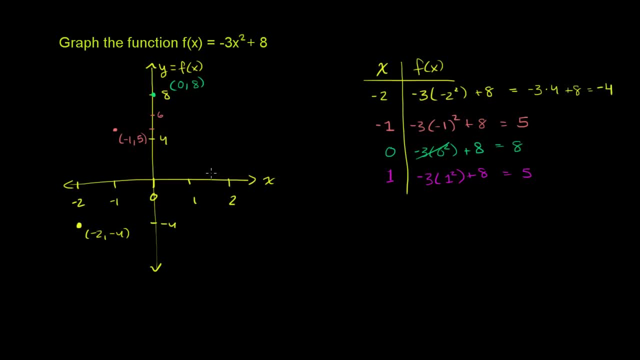 So once again, you get negative 3 plus 8. It is equal to 5.. So this is the point right over here: It is 1 comma 5.. And then, finally, let's do one more point. Let's see what happens when x is positive 2.. 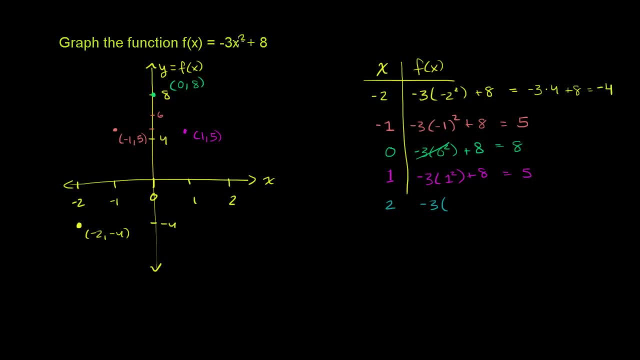 When x is positive, 2, f of x is negative 3.. Negative 3 times positive: 2 squared plus 8.. This, right over here, is negative 3 times 4, which is negative. 12 plus 8 is equal to negative 4.. 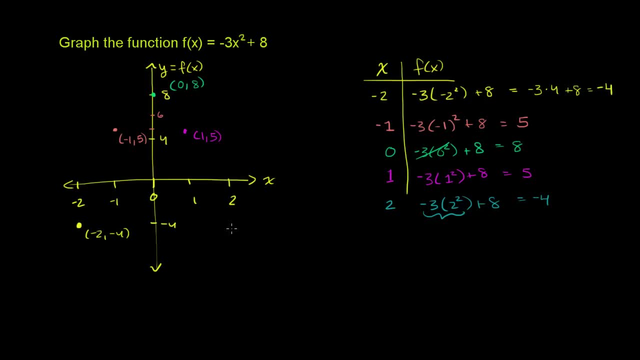 So when x is positive 2, y equals f of x is equal to negative 4.. So this over here- and you might want to plot even more points to get the general shape of it- is going to be a downward opening curve. 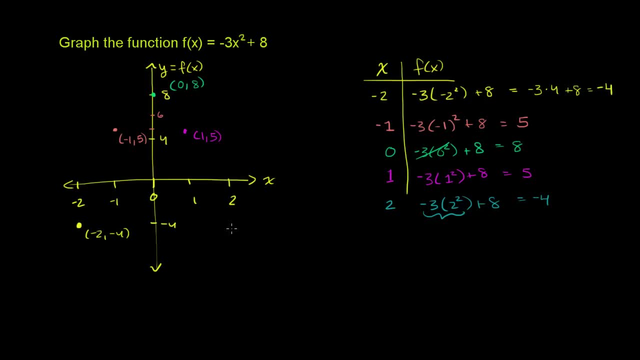 So when x is positive 2, y equals f of x is equal to negative 4.. So this over here- and you might want to plot even more points to get the general shape of it- is going to be a downward opening curve. 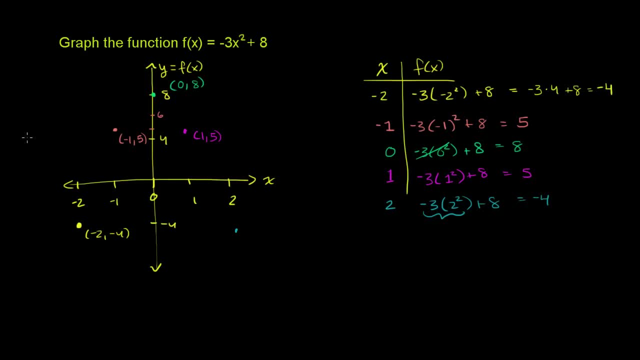 a downward opening- parabola, we could call it- And it will look like this, And I'll draw it as a dotted line Just so that I can do a decent job of it. It's going to look something like this: curve. 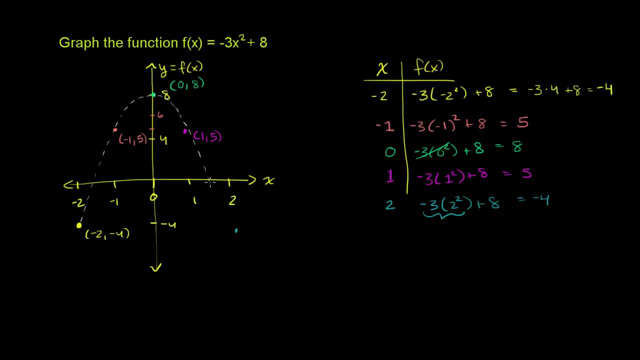 I think the main thing is, I have my scale off a little bit, So it's going to look something like that, And so this point is right over here. I'm going to have to make these points a little bit bigger, so they fall out of my line. 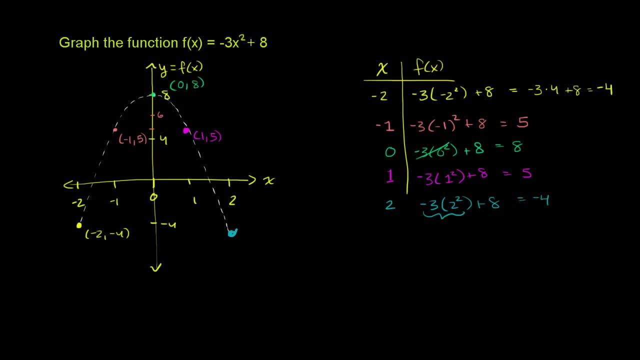 But I want the curve to look somewhat reasonable. So this point is right over there. And this last blue point is the point 2 comma negative 4.. And if you're saying wait, how do you know to curve it just like that, using those points? 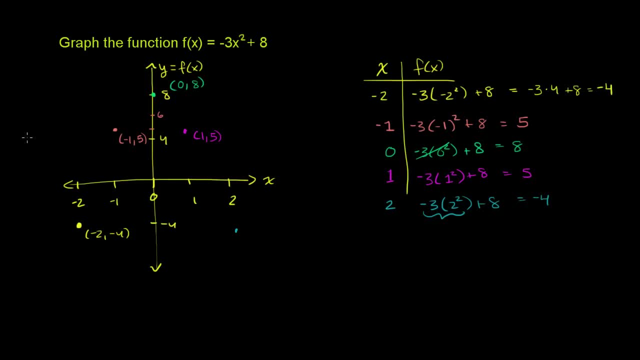 a downward opening- parabola, we could call it- And it will look like this, And I'll draw it as a dotted line Just so that I can do a decent job of it. It's going to look something like this: curve. 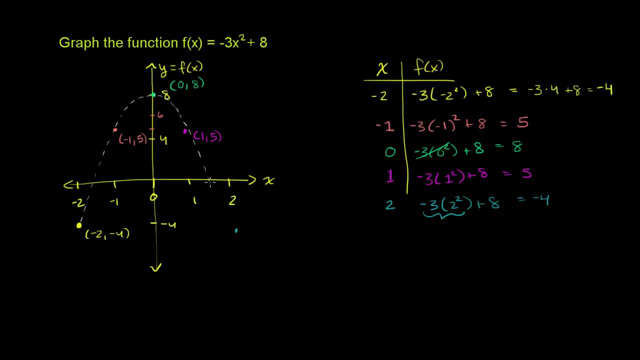 I think the main thing is, I have my scale off a little bit, So it's going to look something like that, And so this point is right over here. I'm going to have to make these points a little bit bigger, so they fall out of my line. 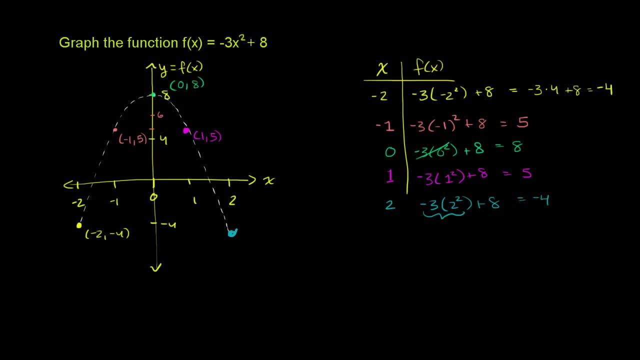 But I want the curve to look somewhat reasonable. So this point is right over there. And this last blue point is the point 2 comma negative 4.. And if you're saying wait, how do you know to curve it just like that, using those points? 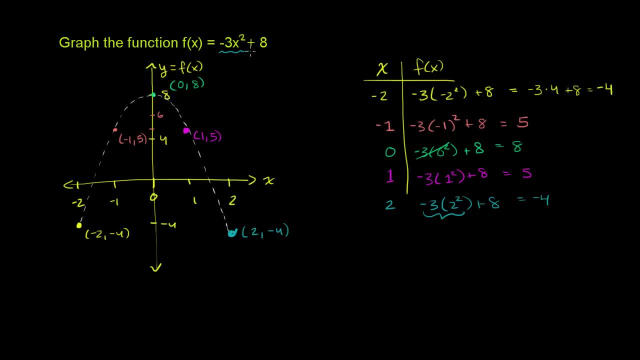 Frankly, that's just from previous experience, knowing that this is a parabola. If you really wanted to verify it for yourself, I really encourage you to take out some nice, clean graph paper and plot the points exactly, And then you could even try points like negative 1 half.